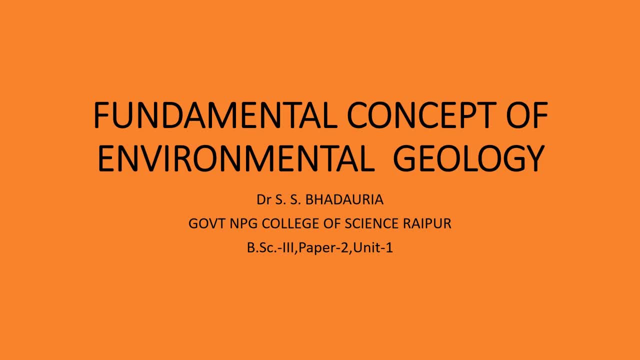 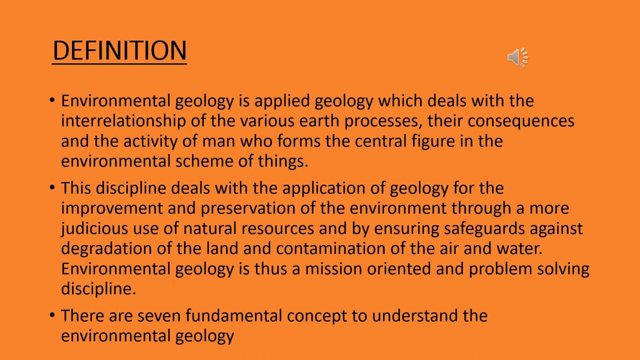 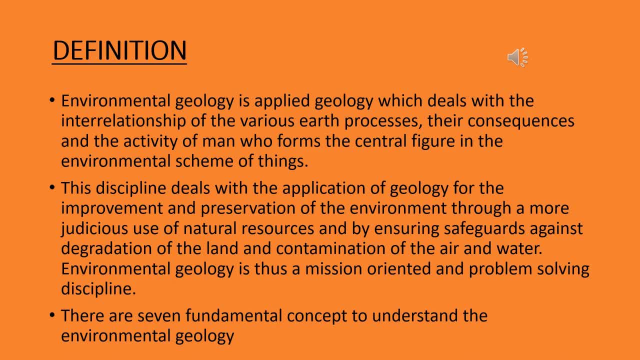 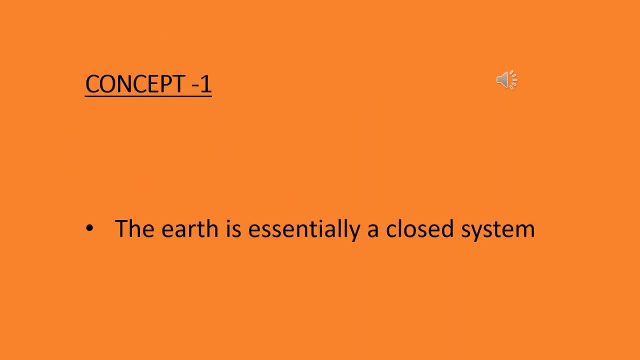 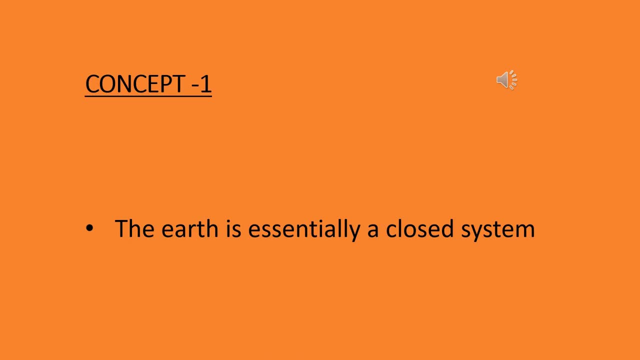 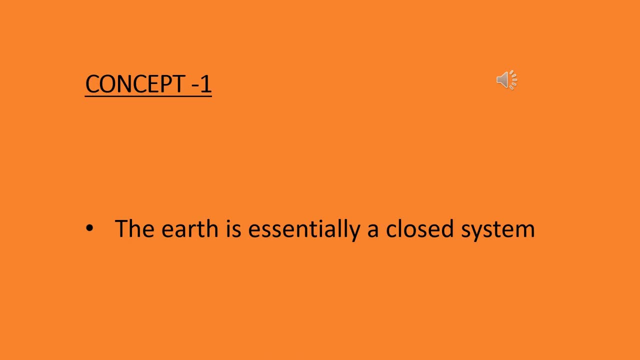 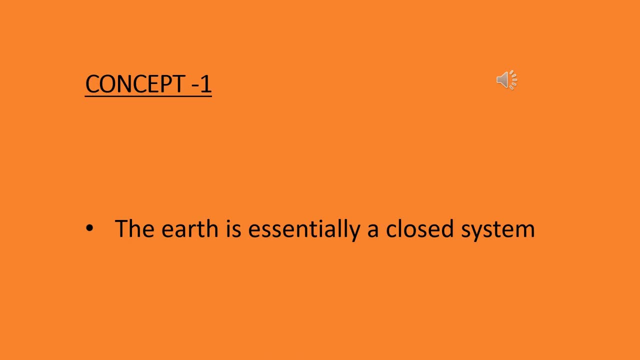 If there is a change in the intensity and frequency of the activity in one part, the intensity and frequency of the activity in the other part changes. That is, if there is any change in the atmosphere related to the atmosphere, whether it rains or not, then there will be a change in the lithosphere of the earth, its effect will be there, the effect will be there in the biosphere, the effect will be there in the androsphere. In this way, the process of change in one part of the natural environment and change in the other part is called the principle of environmental unity. The earth can be seen as a closed system, a rock cycle, a water cycle, for example, in which the materials are recycled or recycled. 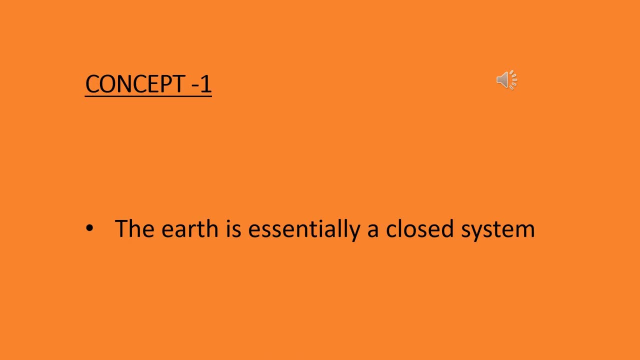 Since the natural resources of the earth are limited, we need to understand the nature of the earth. We need to understand the nature of the earth. Therefore, it is necessary to know the intensity and frequency of those activities that are responsible for it. 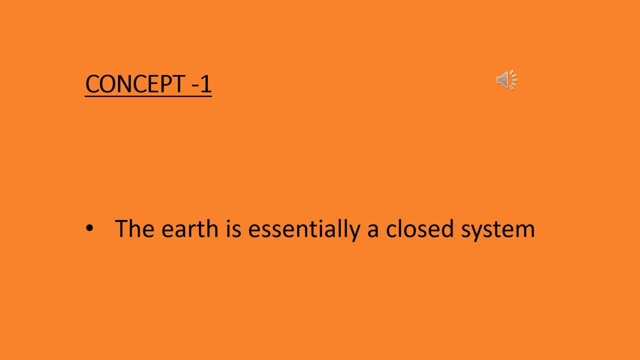 That is, it is necessary to know those activities that they are recycling. 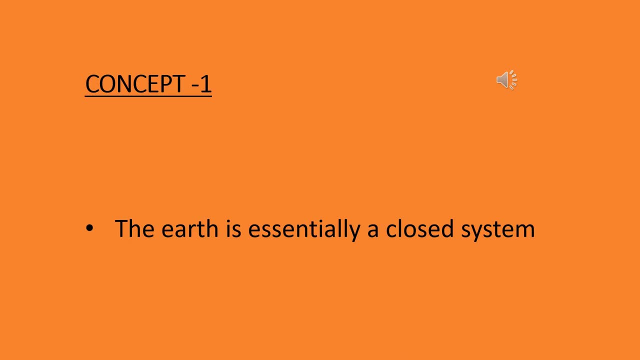 For example, if we have to manage the water resources of a place, then we need to know the nature and limits of the natural activities of that place, which are responsible for the availability of fresh and fertile water in that place. That is, it is necessary to know the nature and limits of the soil. For example, if we have to manage the soil resources of the ewe in that place, then we have to know the nature and the limits of the soil, which are responsible for its survival and the ability to grow. That is why we need to know the nature and the limits of the soil. Concept two. 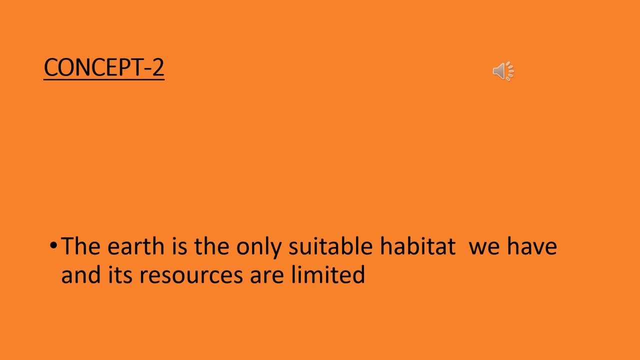 The Earth is the only suitable habitat we have, and its resources are limited. Concept two. The Earth is the only suitable habitat we have, and its resources are limited. That is, the whole universe, the earth only has the means of living on the basis of the facts we know, and the availability of the available resources has enabled human development. 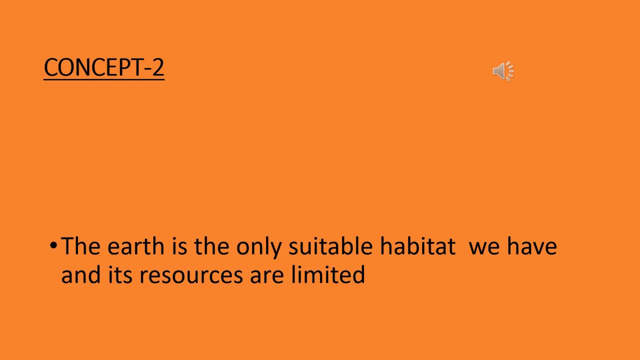 But these resources are limited. Some of the available natural resources can be re-produced. These are called renewable resources. Like padav jagat, you can plant a lot of plants, you can grow grains, you can plant forests. 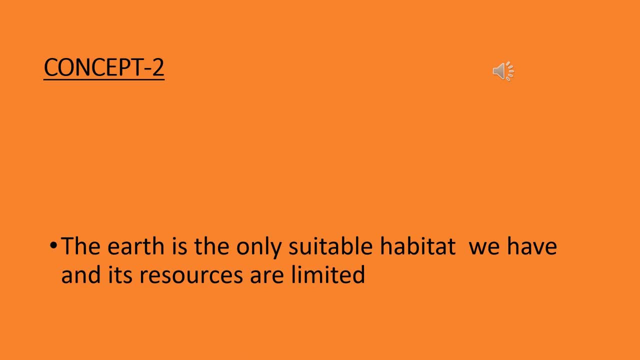 But there are a lot of resources that cannot be re-produced. This is why it is important today that the resources obtained from natural resources be re-produced or recycled on a large scale. In the future, they will be deficient due to the lack of population growth and the lack of resources. We will definitely feel a shortage of these natural resources. And this shortage will have a negative effect on the environment. A small amount of useful minerals will be used. To achieve this, a large-scale mining process will be carried out, which will continue to disrupt the balance of the environment. And the existence of plants and living beings will also be in danger. The evidence obtained from the geological history of the earth tells us that the number of extinct species is much higher than that of the living. 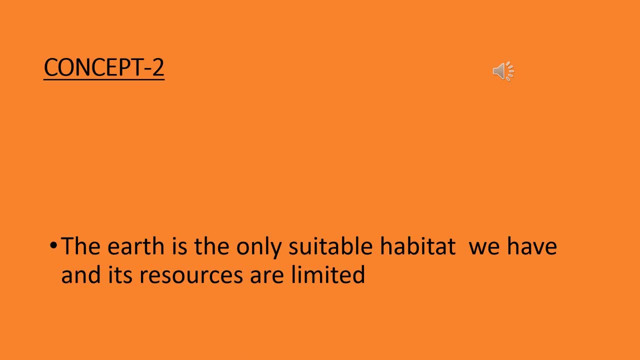 By taking education from this fact, humans should try to balance the environment. Otherwise, the human race will also become a science of the earth. In the history of geoscience, the index will be registered as a fossil. The students who study geoscience understand this very well. Concept 3 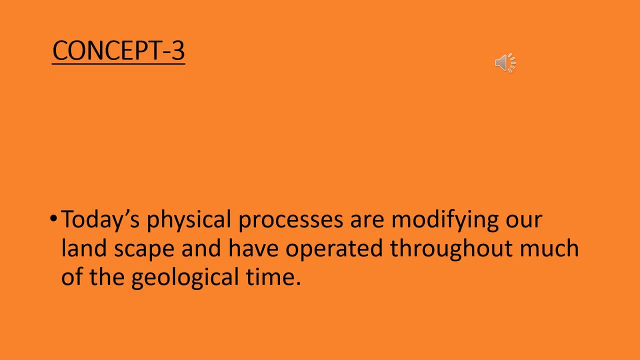 Today's physical processes are operated throughout geological time and modifying our landscape. The current geoscientific processes are derived from ancient geoscientific times, which is why the earth's current geoscience is formed. The intensity and intensity of these geoscientific processes has been changing dramatically in nature. 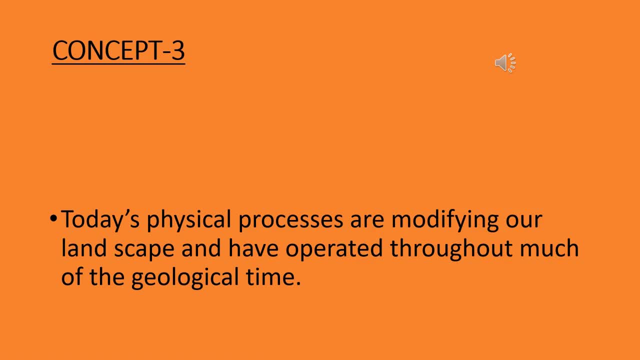 In this regard, it is very important for us to understand the processes of humans, due to which the intensity and intensity of geoscientific processes are changing. For example, the intensity of a flood is either less or more than that of human processes. For example, by making a dam, we reduce the probability of a flood. On the other hand, by putting obstacles in the natural ecosystem, we also create a situation of a flood. Therefore, it is very important for us to know how our processes will affect natural processes in the future. It is also true that in comparison to natural geoscientific processes, human processes will be very small in the global context. Concept 4 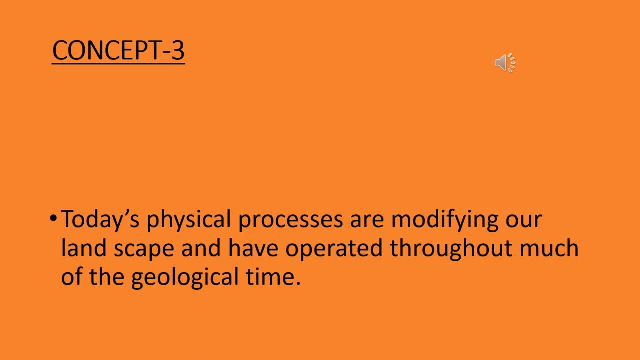 Land slide is another incidence which indicates the human interference. 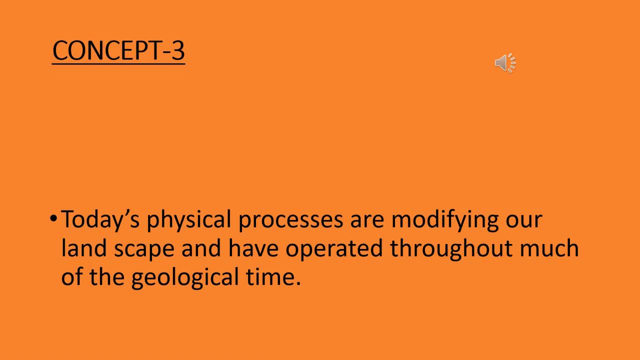 That is, an example of the increasing occurrence of landslides or earthquakes. Concept 4 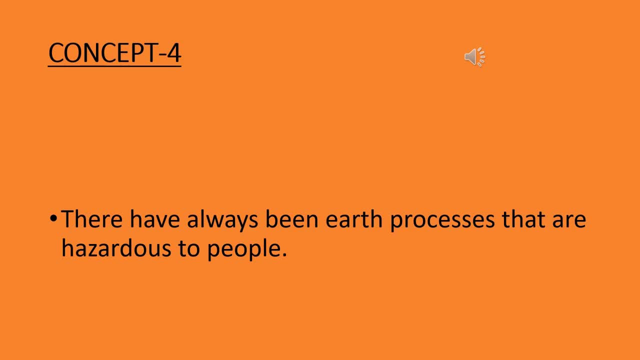 There have always been earth processes that are hazardous to people. There are many such processes in the earth. There are many such natural processes that are hazardous to humans, such as a flood, earthquake, tsunami, earthquake, flood, etc. It is not possible to prevent these natural processes, but by recognizing the coming disasters, its impact can be reduced, so that the biosphere reaches at least 6, and the environment remains safe. 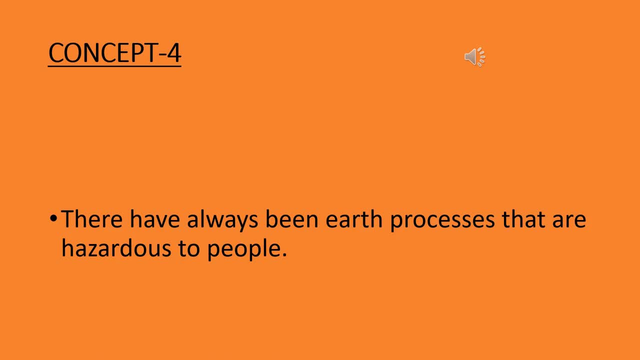 For this, science has progressed so much, that we can predict the correct timing of these natural processes, or at what time such disasters are going to occur, and to a certain extent, we can present its information by analyzing it. 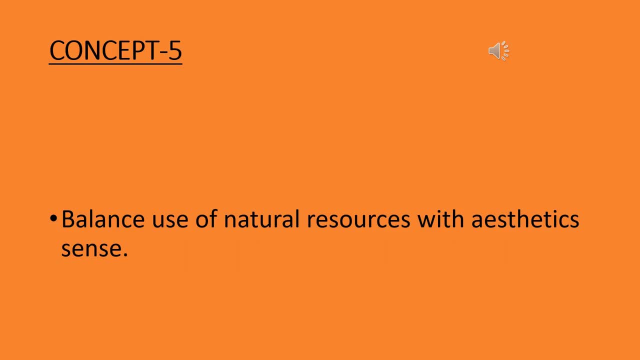 Concept 5 Balance use of natural resources with aesthetic sense. The resources available on earth, such as water, land, etc., should be used to make such projects, which also lead to economic development and natural beauty, which will continue to advance the tourism industry of that country. 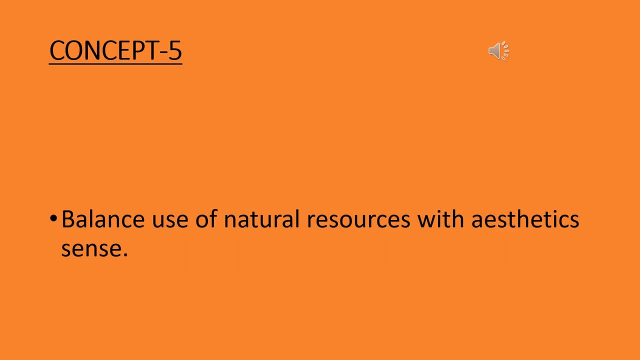 In the present, natural beauty is also considered as a resource. Therefore, in order to develop any such project, it is very important to keep in mind this principle of the environment. 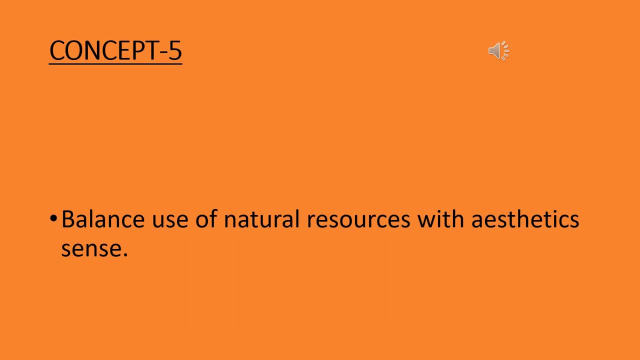 Concept 6 There are many countries in the world, whose economic status depends on tourism. 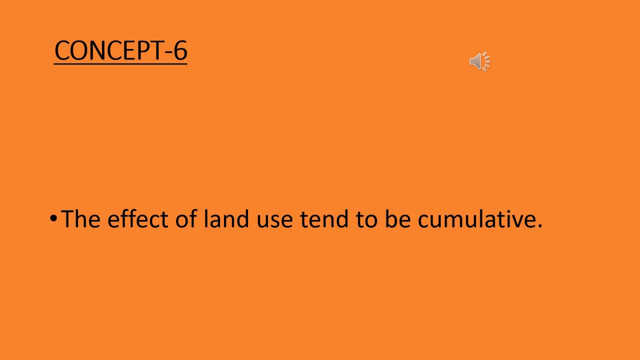 Concept 6 The effect of land use tends to be cumulative. 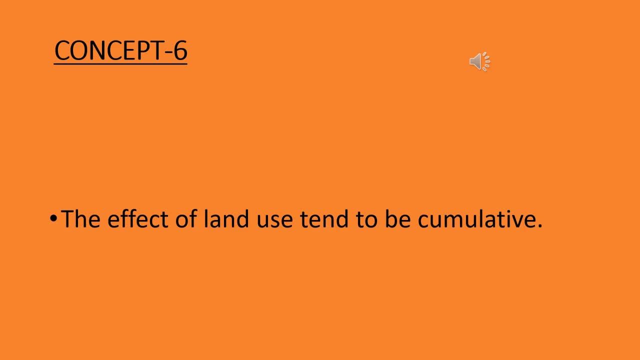 The way land has been used by humans, its effect is visible to the generations to come. 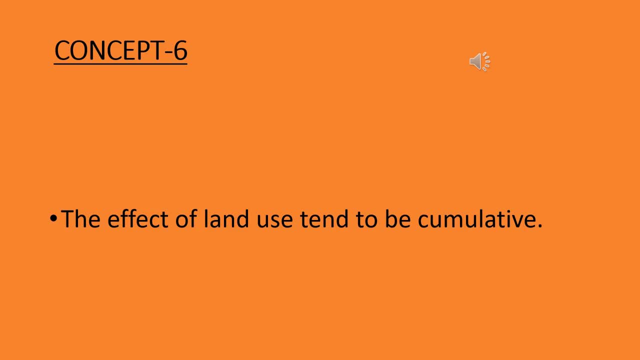 For agriculture, the need for land was the first event, This was the first event that started affecting the environment. Along with the development of agriculture, such systems began to develop in which humans began to live in one place, which started to have a negative effect on the resources, environment and the environment of that place. So, how do we use the land? This has to be seen in historical context. Along with the development of the environment, in about 15,000 years, humans have changed the entire surface of the earth. 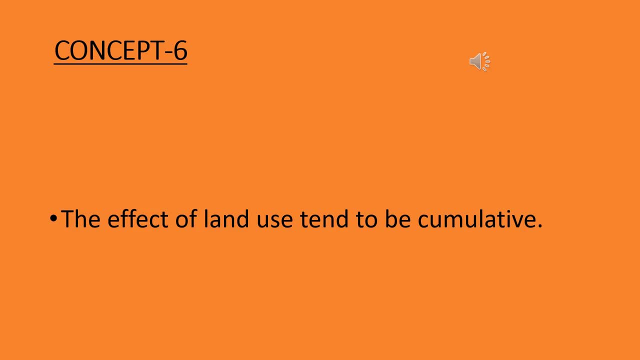 This process is in progress at high speed. Concept 7 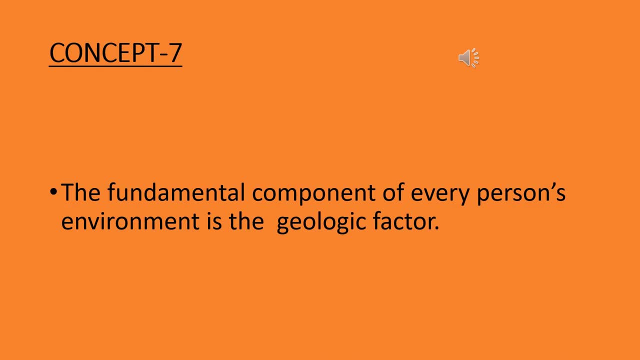 The fundamental component of every person's environment is the geologic factor. This is the last example and it is said that to understand the environment, it is necessary that we should understand the environment. The knowledge of geoscience and the branches of other related sciences is necessary. The creation of this principle is due to the fact that geoscience is directly related to the environment. 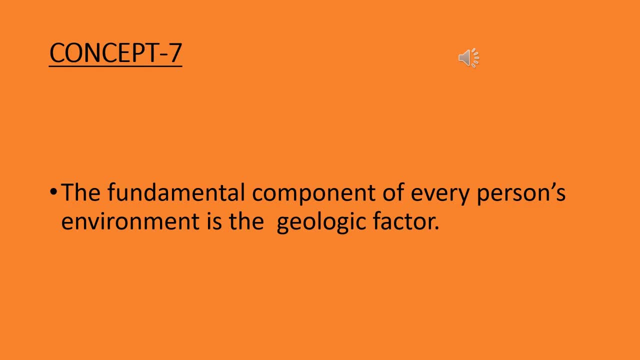 And since we live on the surface of the earth, it affects geoscientific processes either experimentally or unnecessarily. 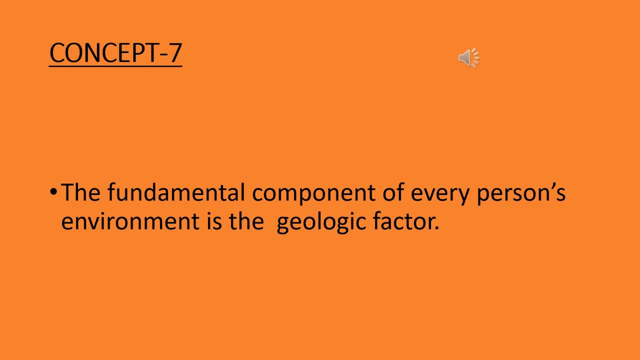 Therefore, to understand our complex environment, it is necessary that we should understand the various subjects of geoscience, such as geomorphology, petrology, sedimentology, tectonics, and hydrogeology, economic geology, engineering geology, etc. Apart from this, a geoscientist should also be familiar with the research on the environment in other fields of science, such as biology, environmental law, architecture, engineering, and physical, cultural, economic, and urban geography. In this way, environmental geoscience is a very interrelated science. It is necessary to understand the environment. Concept 8 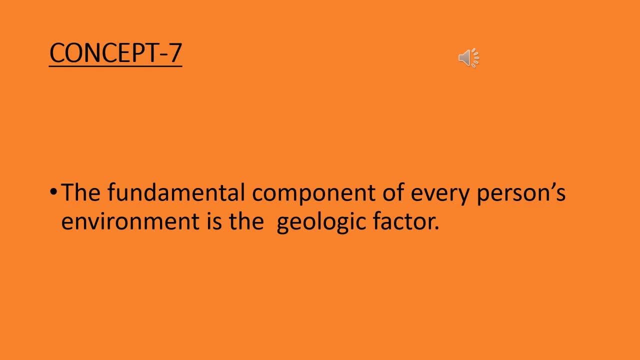 Geoscience is a very interrelated subject in which the knowledge of other subjects of science and social subjects is very important. 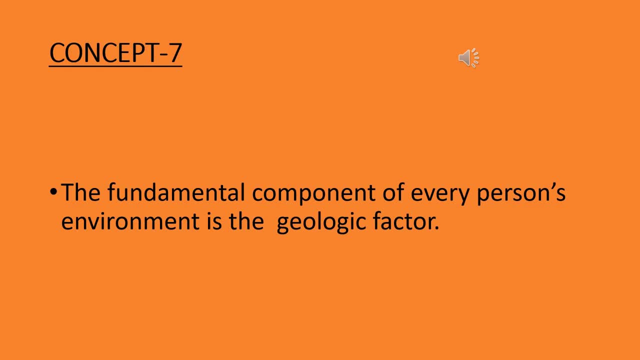 This fact becomes even more evident when we start studying environmental issues.